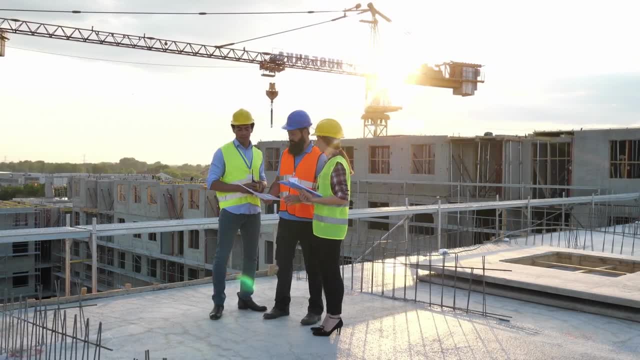 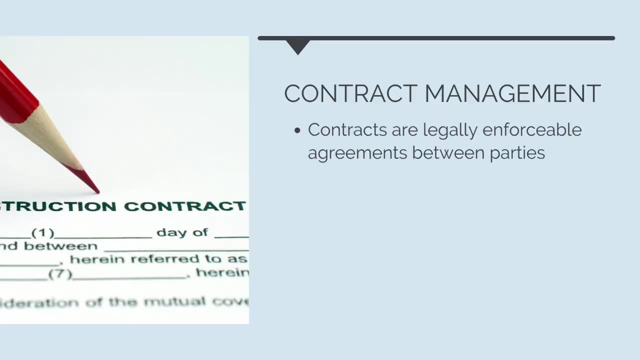 Construction projects are massive exercises in teamwork. We need ways to work together with other companies. That's where contracts come in. Contracts are legally enforceable agreements between parties. They are an essential part of construction management because contracts define the relationships between all the parties that come together to deliver a construction project. 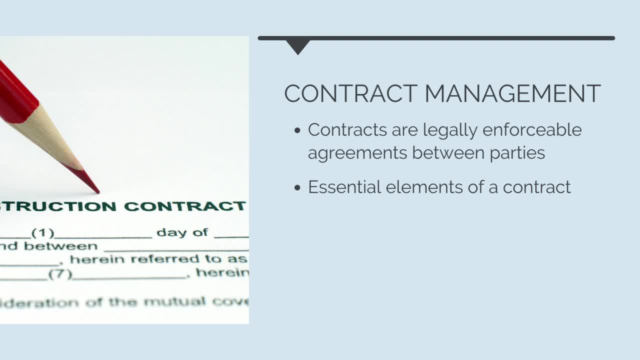 To effectively use construction contracts, we need to understand the essential elements of a contract. The two key types of contracts we deal with are the head contract, which is the contract between the client and the general contractor, and subcontractors, The contracts between us and 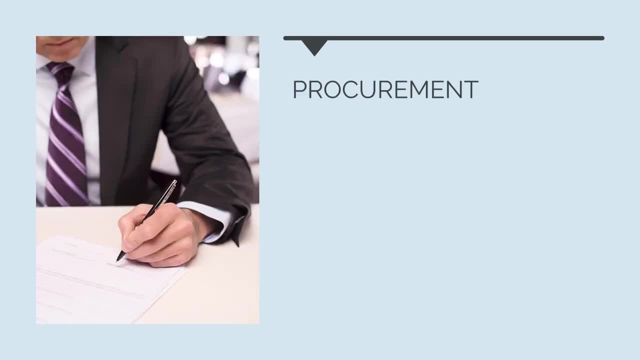 our supply chain. Procurement is closely related to contract management. Procurement is the process of finding and acquiring the external goods and services needed to deliver a project. For us, the general contractor, this means finding and signing subcontract agreements with all of the 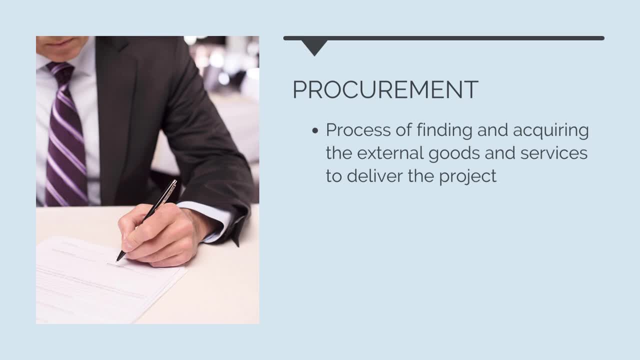 subcontractors and suppliers. we need to complete the project scope. This occurs in two stages: planning and executing procurement. Planning procurement requires us to work out what we need to procure. It involves a lot of work. It involves a lot of work. It involves a lot of. 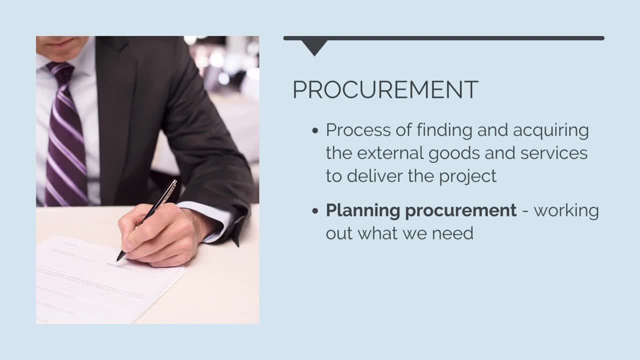 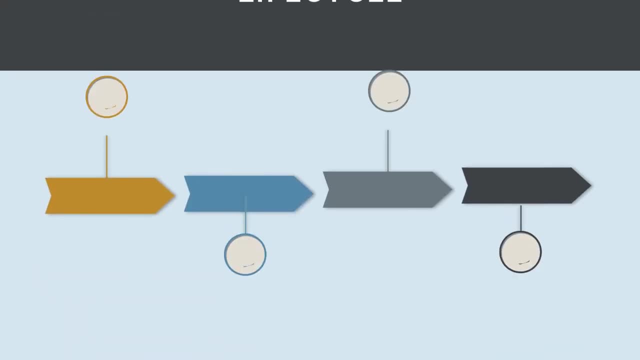 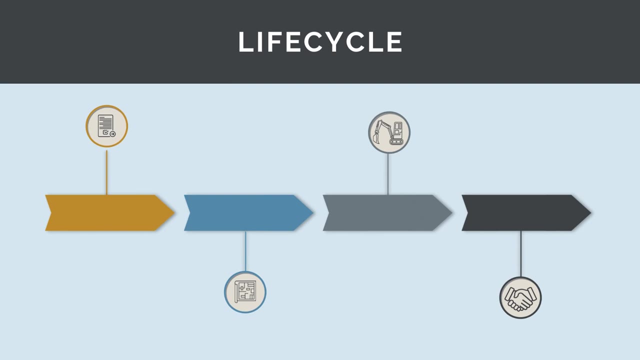 work. It involves developing the procurement strategy and working out what subcontractors we need. Executing procurement is then the process of creating tender packages, running tenders and awarding subcontracts. As with all the other construction management skills, procurement and contract management is used across the life cycle of a construction project. In the work, 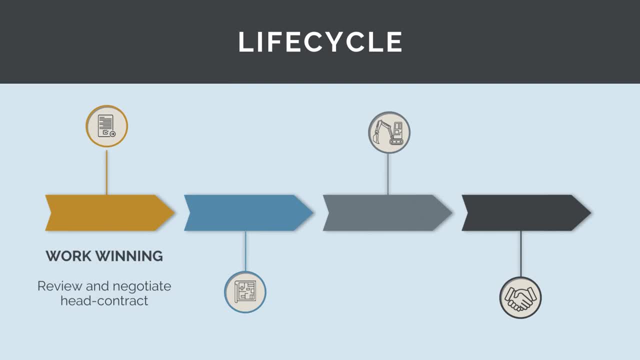 winning phase we will review and negotiate the head contract with our client. We will also begin some procurement activities as part of developing the delivery methodology and estimate for the schedule. During the pre-design and pre-construction phase we will work out the subcontracts. We will conduct the bulk of our procurement. We will also begin the process of 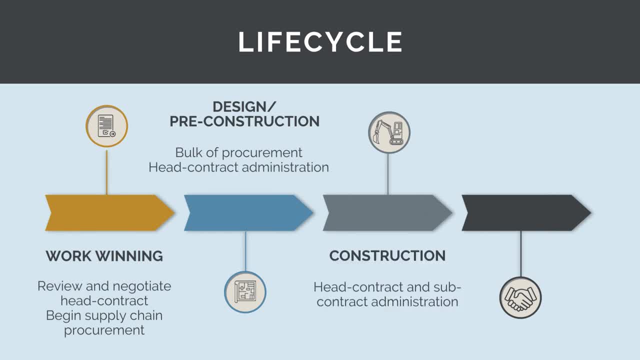 administrating the head contract. During the construction phase, we will administer all the subcontracts and continue administrating the head contract. And finally, in the closeout phase, we will need to close out the head contract and all of our subcontracts, The key tools and 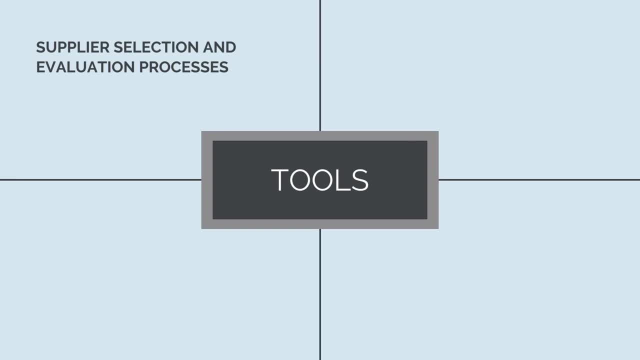 techniques to master this skill are supplier selection and evaluation. develop criteria for supplier selection. conduct competitive bidding processes and evaluate suppliers based on their qualifications, capabilities, pricing and performance. The key tools and techniques to master this skill are supplier selection and evaluation. develop criteria for supplier selection. 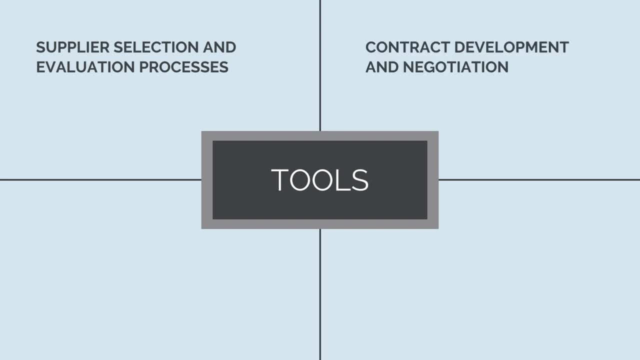 and evaluation, conduct competitive bidding processes and evaluate suppliers based on their qualifications, capabilities, pricing and performance. The key tools and techniques to master this skill are contract development and negotiation. Draft clear, comprehensive contracts that clearly define project requirements, scope of work, pricing, milestones, terms and conditions. Negotiate terms.